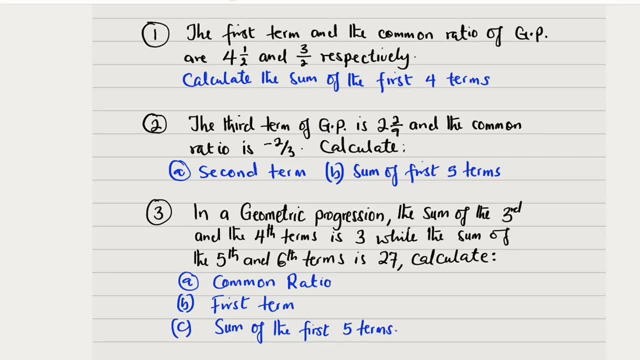 Hello, good day viewers. In this tutorial, we are going to work on three word problem questions. All of these three questions are related to geometric progression series. Therefore, if you are new here, consider subscribing. Press the bell icon so that you will be notified whenever I upload a new content, and don't forget to share to your 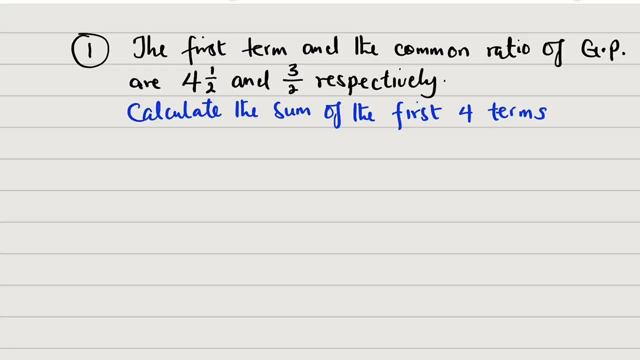 learning colleagues. Alright, here is the first question, which reads: the first term and the common ratio of geometric progression sequence are given as 4, 1 over 2 and 3 over 2 respectively. We are only asked to find the sum of the first four terms. So now let's write our data. 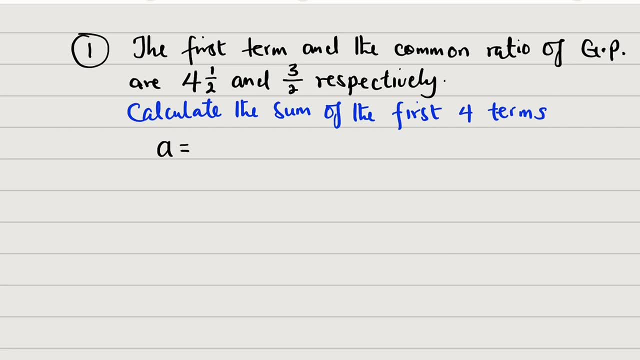 a, which is the first term, is given as 4, 1 over 2, but let us write it in an improper fraction: 2 multiplied by 4 is 8 plus 1 is 9, so we have 9 divided by 2.. 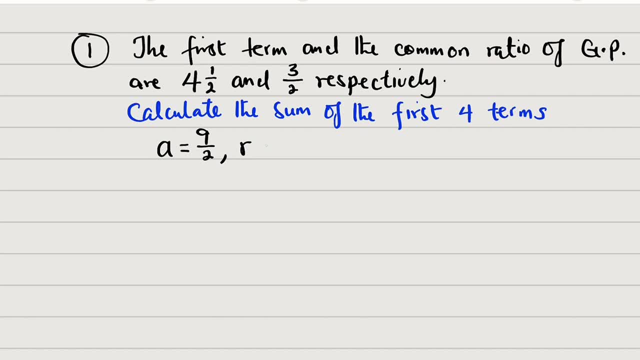 We are also given a roughly 1 over 2, which represents the Id сложation using the develop equation, given the common ratio r as 3 divided by 2.. n from the question is 4.. You can see that r is. 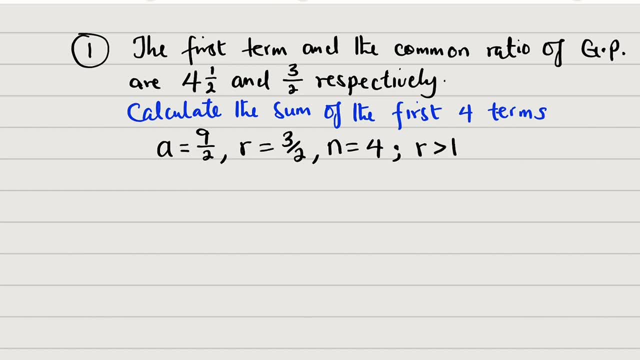 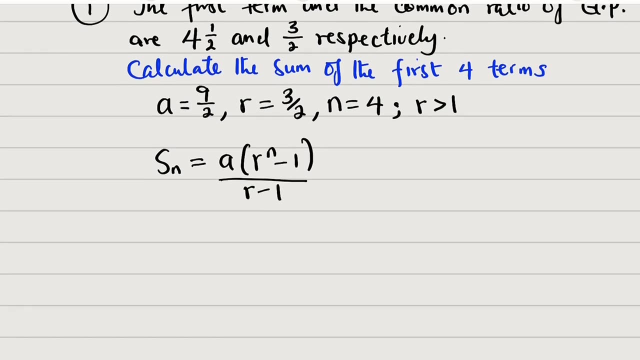 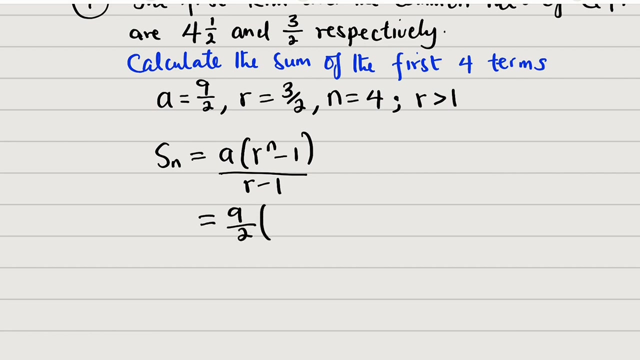 greater than 1.. Therefore, we are going to apply the formula, as n equals a multiplied by r, to the n power minus 1 divided by r minus 1.. This is equal to a is 9 divided by 2 multiplied by r is. 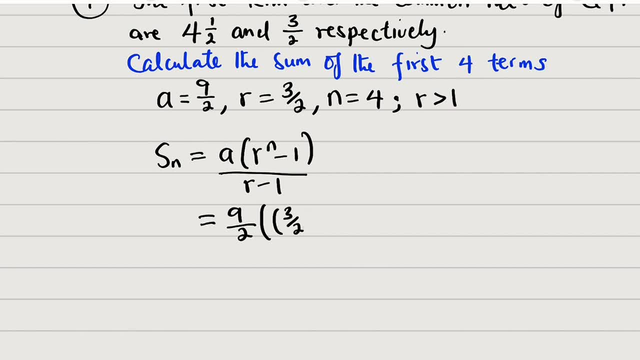 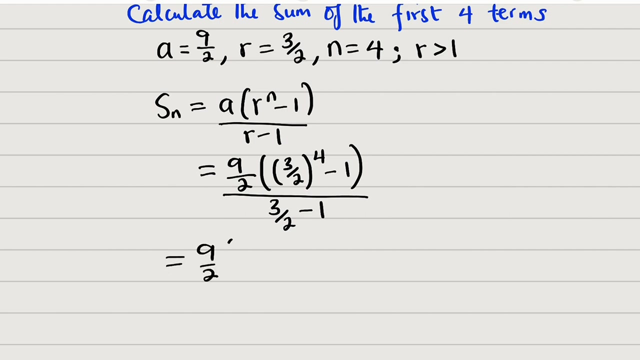 3 over 2 raised to the power of n, which is 4 minus 1.. And all of this divided by r, which is 3 divided by 2 minus 1.. Let's further simplify: This is equal to 9 divided by 2 multiplied by. 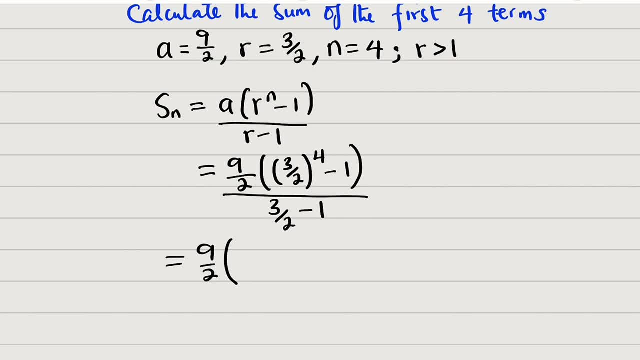 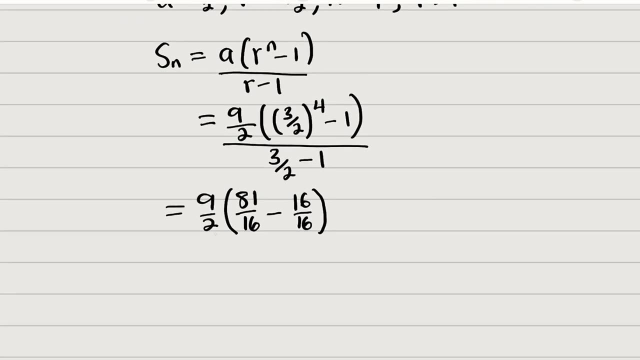 3 to the power of 4 is 81. And 2 to the power of 4 is 16 minus 1.. And this one can be written as 16 divided by 16.. I want to have a common denominator. All of this, divided by r, is: 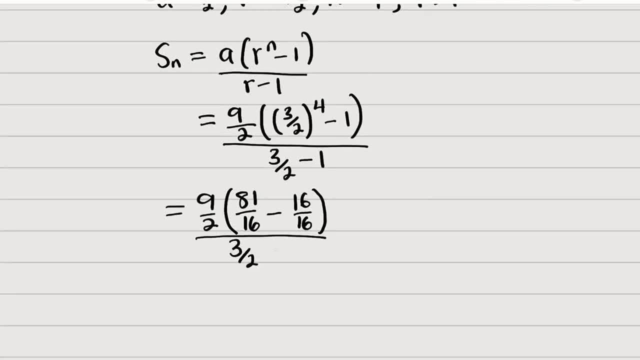 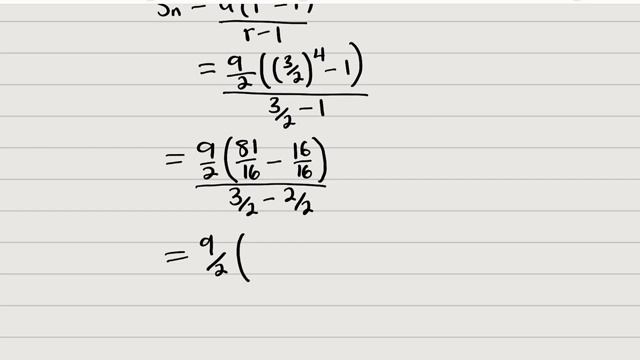 3 divided by 3 divided by 2.. Then minus 2 divided by 2.. I also want to have a common denominator. All right, This is equal to 9 over 2 multiplied by 81. minus 16 is equal to 65. So we have 65. 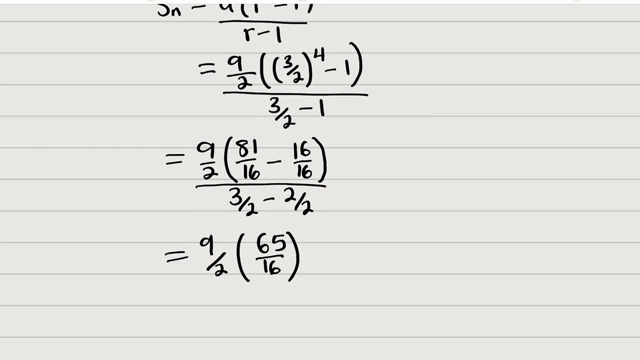 divided by 16, divided by 1 over 2.. Okay, This 2 will multiply this 1 over 2. And that is equal to 1.. So we only have 9 multiplied by 65 divided by 16.. And 9 multiplied by 65 is the same thing as 585.. 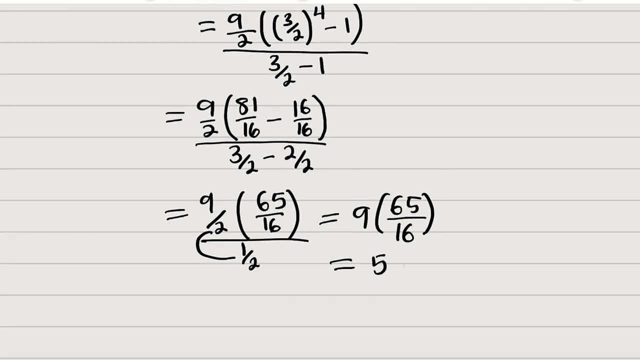 So we have 585.. 585 divided by 16.. This is our final answer, But if you like, you can write it in a mixed number as 36, 9 over 16, because 16 can go into 585, 36 times, with a remainder of 9.. 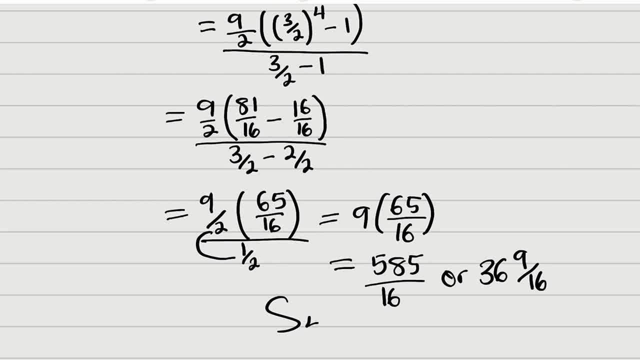 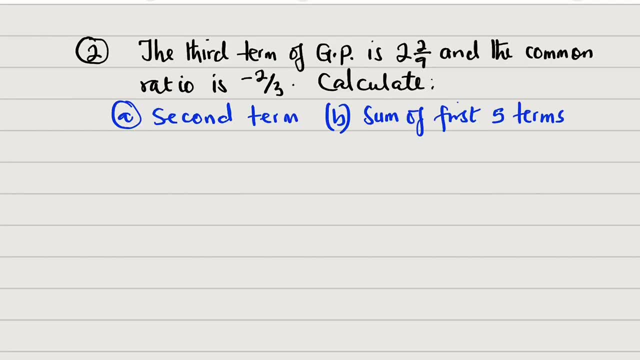 And therefore this is said to be the sum of the first four times. Now let us move on to question number two. Okay, Here is the second question that reads: the third term of GP is 2, 2 over 9, and the common ratio is negative: 2 over 3.. 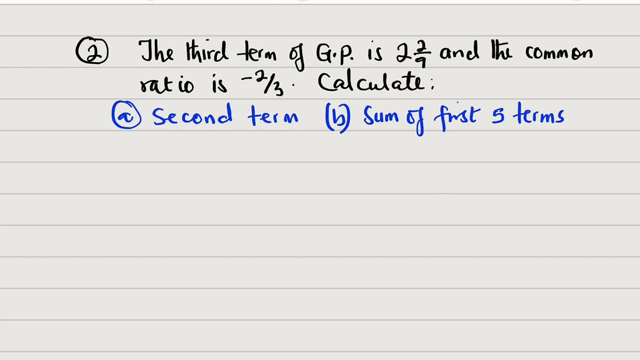 We are asked to calculate the second term and the sum of the first five times. Okay, Let us start with the first one. So for a part, we are given term number three from this question and also the common ratio. So let me write them. 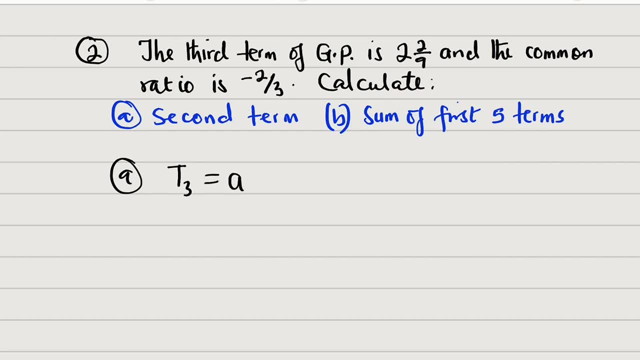 So the common ratio is given from question number three, which is also the same thing as AR, to the second power. It is given from the question as 2, 2 over 9, which is the same thing as 20 divided by 9.. 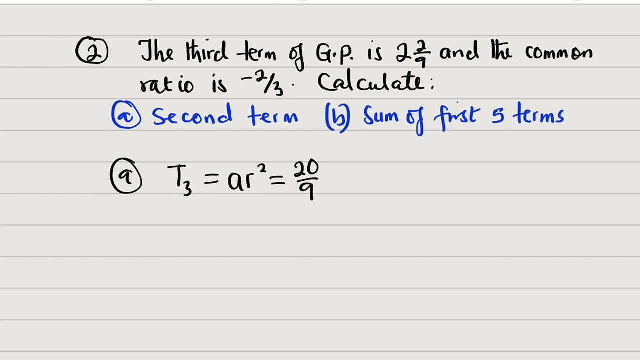 If you multiply 9 by 2,, you get 18 plus 2 is 20.. All right. And also the common ratio is given as negative: 2 over 3.. So now let us use this information to find A, Which is the first term. we can plug R into this equation to obtain A. 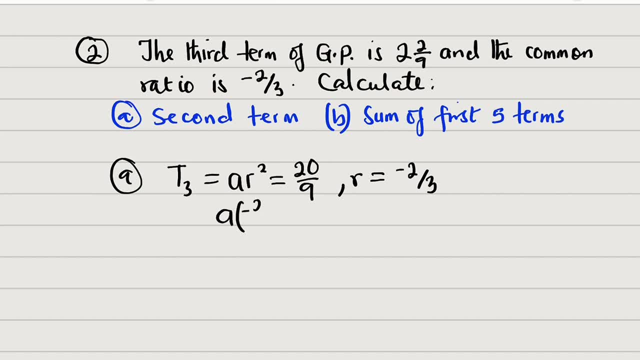 So we have A. R is negative, 2 over 3, and the whole of this. it must be equal to 20 over 9.. All right, This one has a square. A multiplied by 4 over 9 is equal to 20 over 9.. 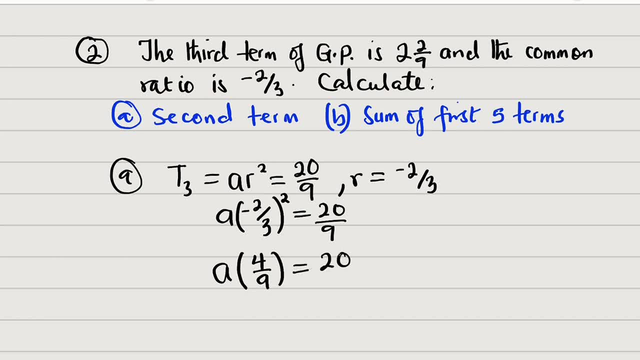 A multiplied by 4 over 9 is equal to 20 over 9.. A multiplied by 4 over 9 is equal to 20 over 9.. We can multiply both sides by the reciprocal of 4 over 9 to get the value of A. 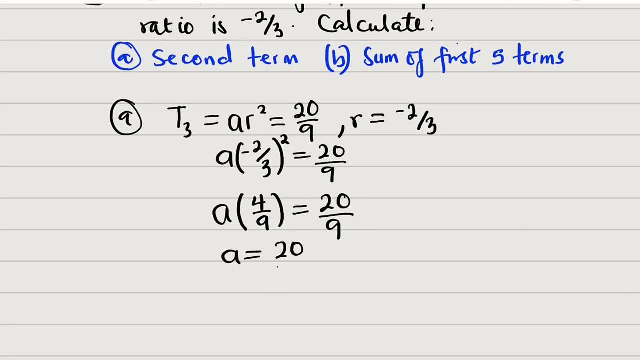 Therefore, A is equal to 20 divided by 9, multiplied by 9 divided by 4.. From here, 9 will cancel 9, and the 20 divided by 4 is equal to 5.. Therefore, A, which is the first term, is equal to 5.. 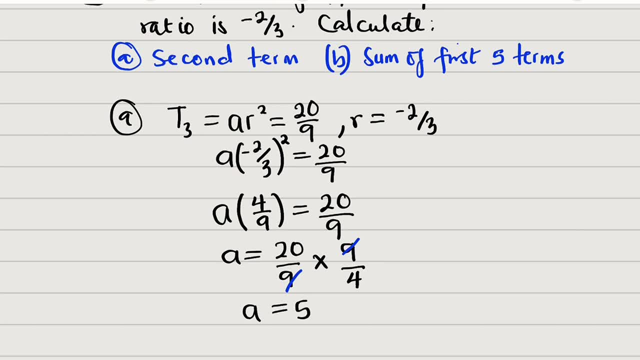 All right, Remember we are looking for the second term. Therefore, let me come here and do that Second term, which is T2, is equal to AR. Therefore, A is 5 and R is negative 2 over 3.. 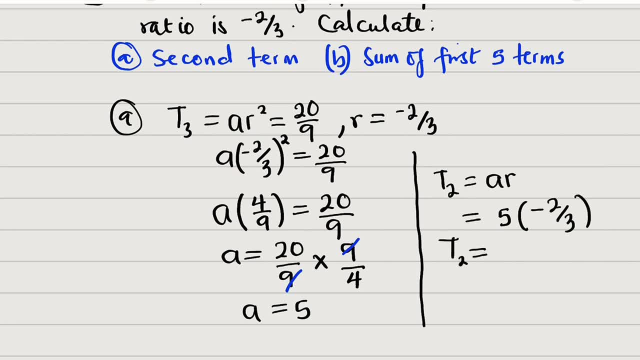 Finally, term number 2 will be equal to negative 2 over 3.. All right, So we have negative 10 divided by 3.. But if you like, you can write it in mixed number as negative 3, 1 over 3.. 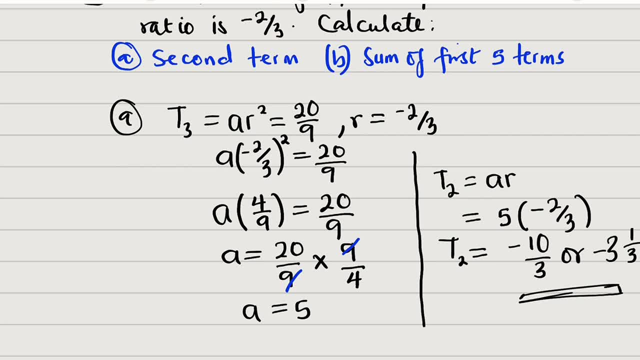 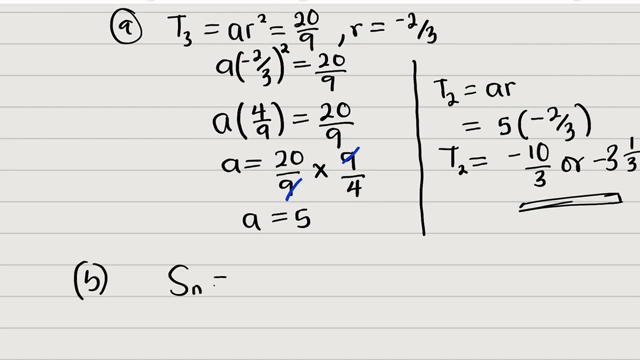 And hence this is said to be the second term. But we are also asked to find the sum of the first five terms. So B part This N is equal to A, multiplied by Y is R, R is negative. So we are going to use this formula. 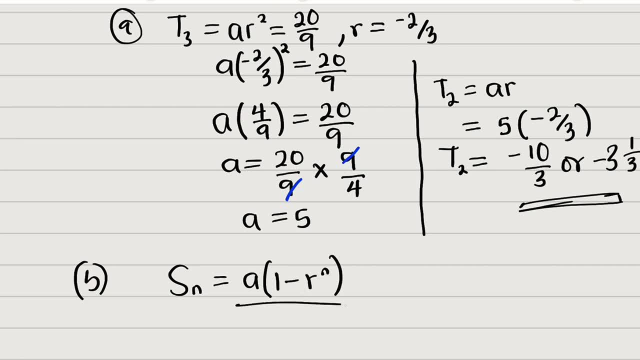 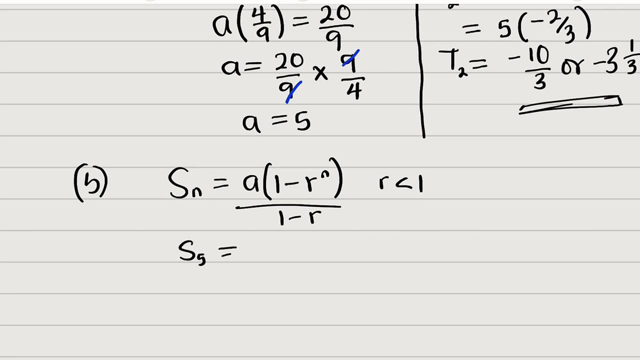 1 minus R to the N power divided by 1 minus R when R is less than 1.. So let's substitute: N is equal to 5.. As 5 is equal to, A is 5.. You can see it here. 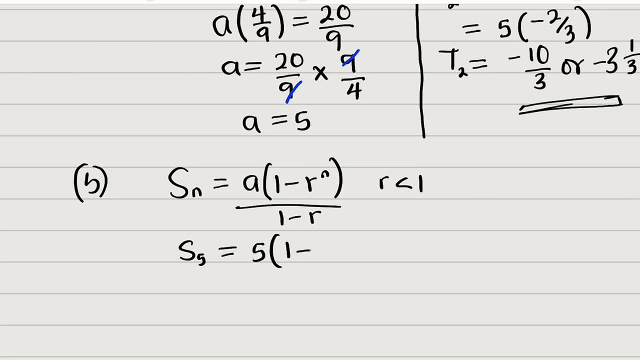 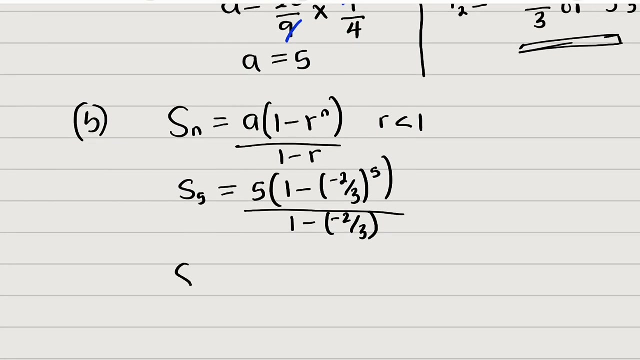 You have. 5 multiplied by 1 minus R is negative 2 over 3, raised to the power of 5.. Divide by 1 minus negative 2 over 3.. All right, Let's simplify this a little bit, As 5 is equal to 5.. 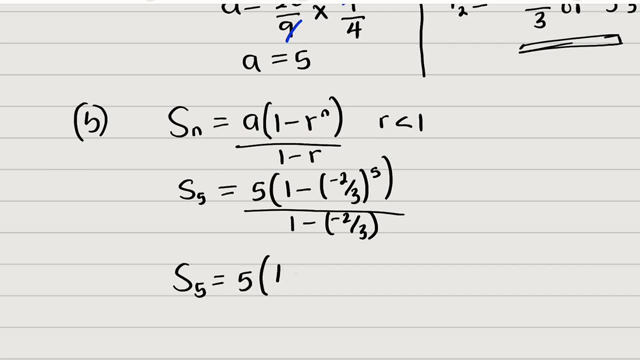 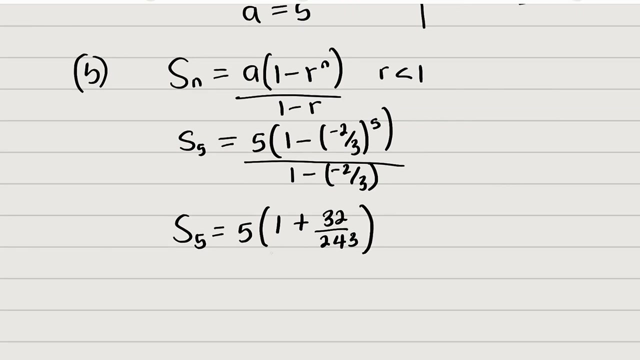 Multiply by 1 plus, Because minus minus will be plus. This is an odd power. 2 to the power of 5 is 32.. Divide by 3 to the power of 5 is 243.. Divide by, We have 3 over 3.. 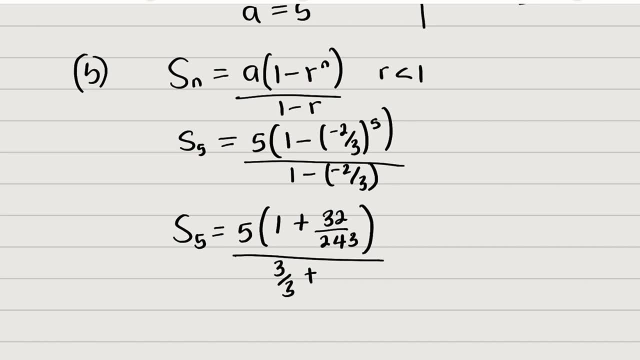 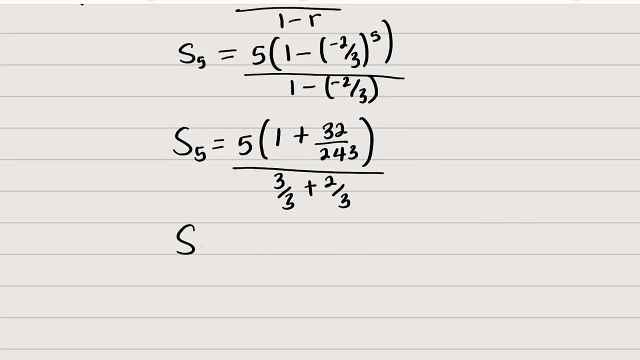 Minus or plus, Let me say, because minus, minus is plus 2 over 3.. Sum of the first five times will now be equal to 5.. I can also write this as 243.. Divide by 243. Just to have common denominator. 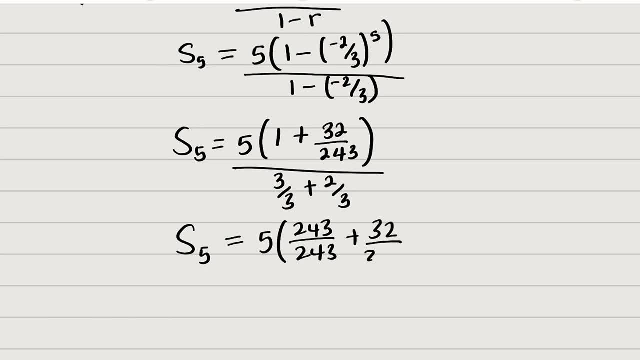 Plus 32. Divide by 243.. 3. Divide by 5 over 3. This 3 can multiply this 5.. We have 15. Divide by 5 is 3.. So the whole of this becomes 3.. 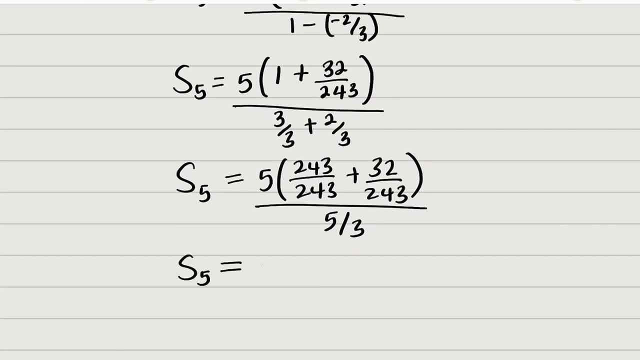 So as 5 is equal to 3.. Multiply by the whole of this, 243 plus 32 will be 275.. So we have 275.. Divide by 243.. This 3 right here can go into 24381 times. 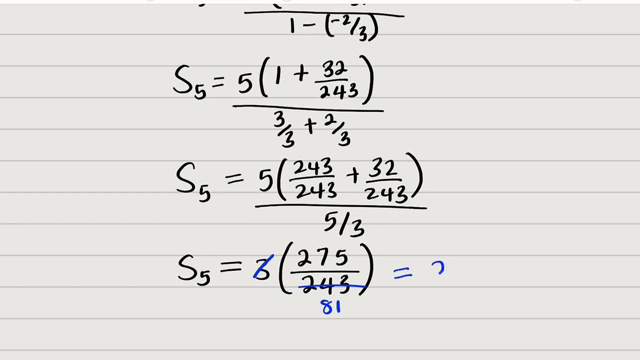 So this is equal to 275.. Divide by 81. And if you like, you can write it in a mixed number, Which is the same thing, Or I can say, or 3, because 81 can go into 275 three times, with a remainder of 32.. 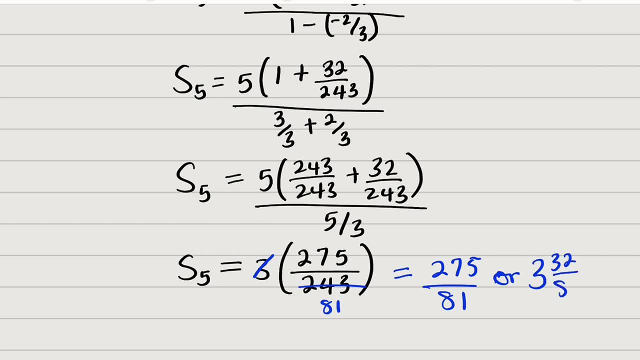 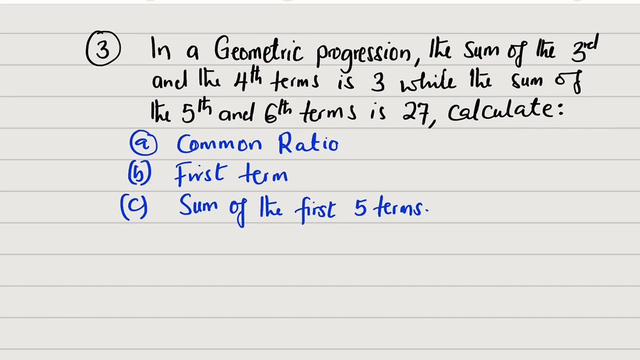 Out of 81. And hence This is the sum of the first five times. All right, Let us move on to the next question. All right, Here is our last question. It says that, in a geometric progression, The sum of the third and the fourth times is 3.. 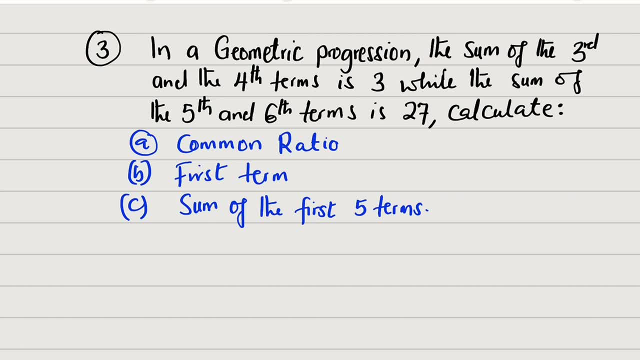 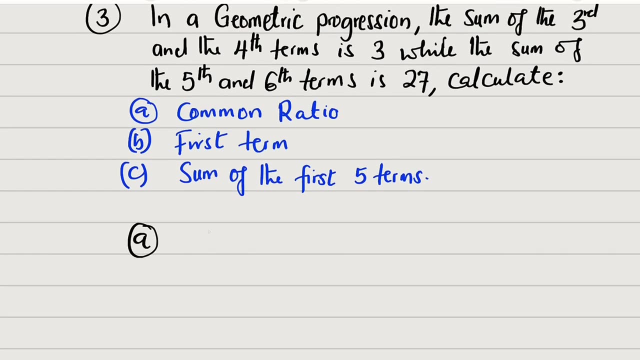 While the sum of the fifth and the sixth times is 27.. We are asked to calculate the common ratio, The first term And the sum of the first five times. Okay, Let us write down our data For the A part, Term, number 3.. 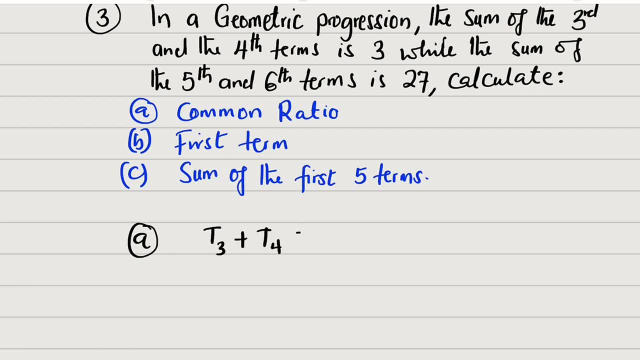 Plus Term number 4. Is equal to 3.. This implies that A R to the second power Plus A R to the third power is equal to 3.. I can bring out A R to the second power. 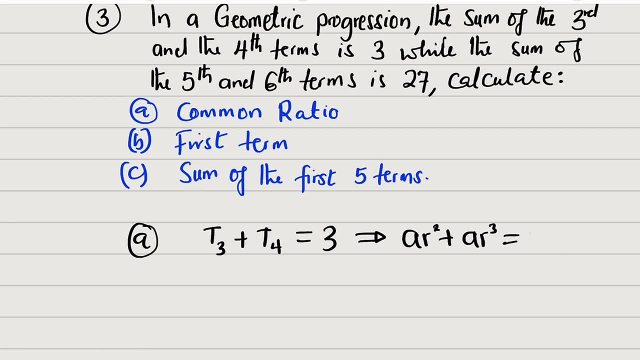 And inside I have one Plus R, And the whole of this Is equal to 3.. Let me call this one Equation 1.. And This is the Equation 1.. Equation 2.. Equation 3.. Equation 4.. 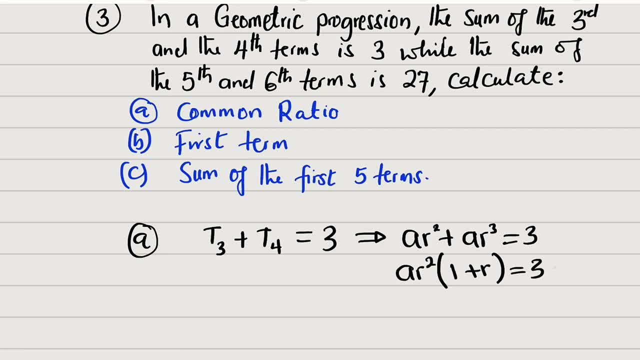 Equation 5. Equation 6. Equation 7. Equation 8. Equation 9. Equation 10. Equation 11. Equation 12. Equation 13. Equation 14. Equation 15. Equation 16. Equation 17.. 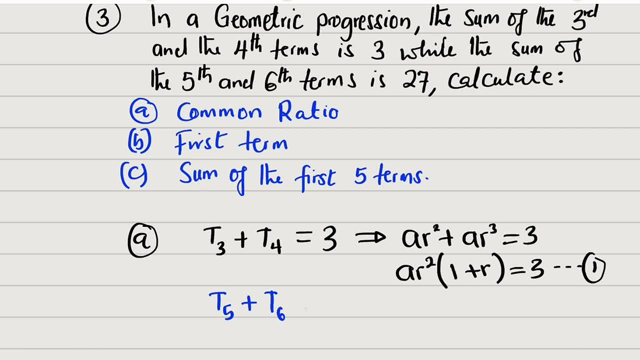 Equation 18.. Equation 19.. Equation 20.. Equation 21.. Equation 22.. Equation 23.. Equation 24.. Equation 25.. Equation 26.. Equation 27.. Equation 28.. Equation 29.. Equation 30.. 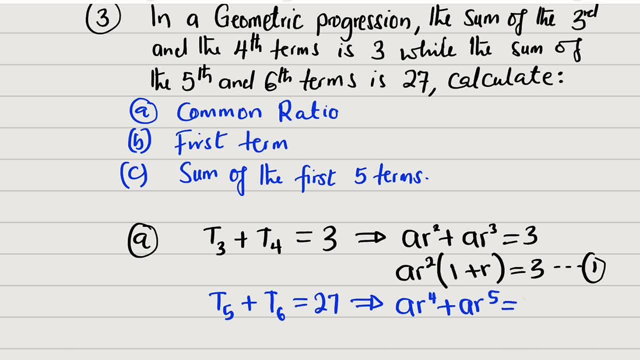 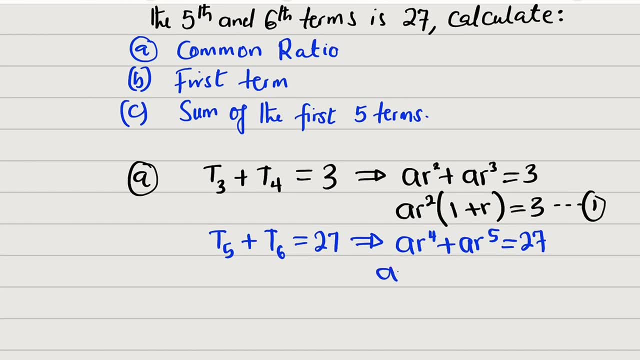 Equation 31.. Equation 32.. Equation 33.. Equation 34.. Equation 35.. Equation 36.. Equation 37.. Equation 38.. Equation 39.. Equation 40. AR to the fourth power, multiplied by 1 plus R, if factorized, this is equal to 27.. 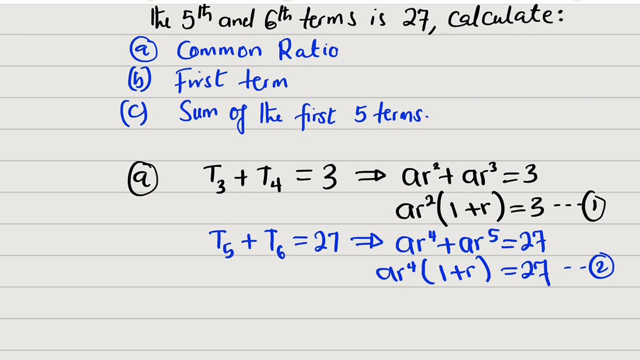 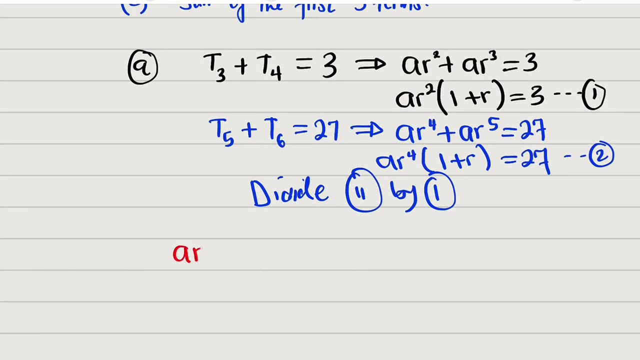 Let me call this one equation number 2.. So now let us divide equation 2 by equation 1.. Equation 2 is AR to the fourth power multiplied by 1 plus R equals 27, and equation 1 is AR to the second power multiplied by 1 plus R, and this is: 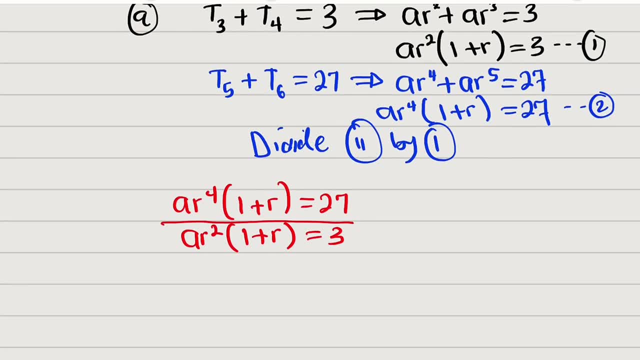 equal to 3.. Okay, from the left-hand side, this A will cancel this. A and R to the fourth power divided by r to the second power is nothing but r to the second power. the whole of this will cancel this, because they are the same and the 27 divided by 3 is 9. this implies that 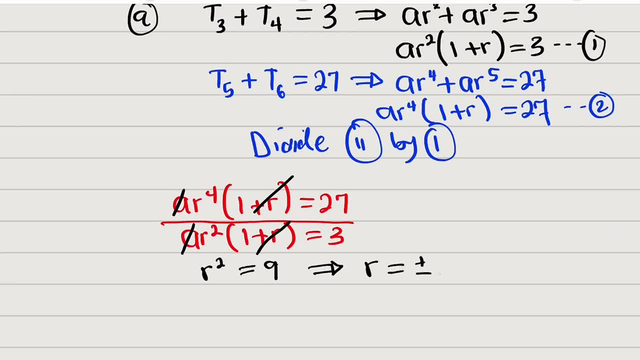 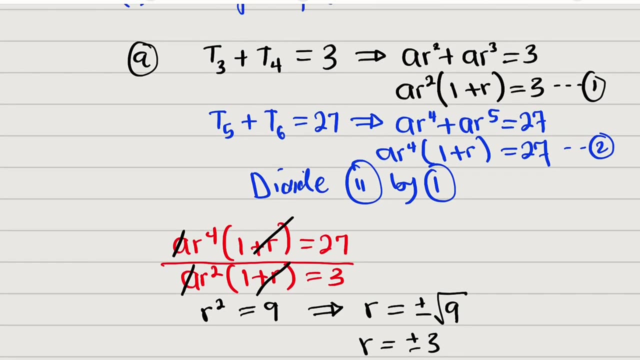 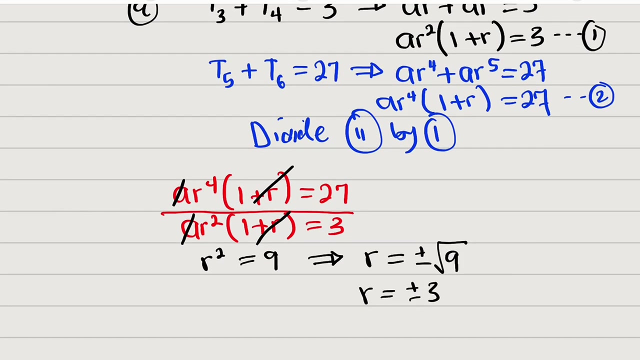 r is equal to plus or minus the square root of 9 and r is equal to plus or minus 3, so the common ratio could either be positive 3 or negative 3. okay, we have answered the a part. the b part said we should find the first term. we can use equation 1, which says that a r squared. 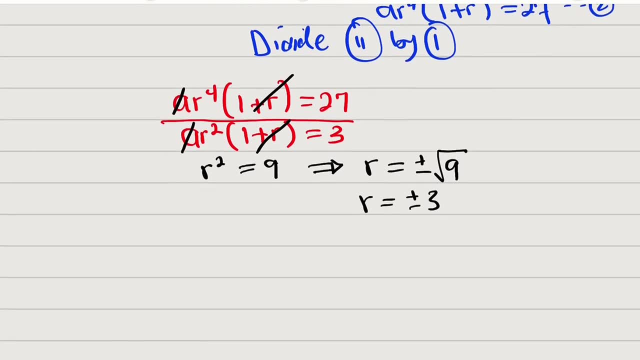 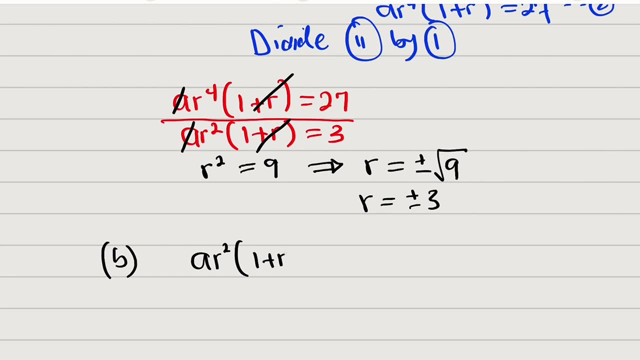 multiplied by 1 plus r is equal to 3. a r squared multiplied by 1 plus r is equal to 3. but i have two r's, one is negative and one is positive. let us first of all apply the positive one. when r is equal to 3, we have a r which is 3 to the second power, then 1 plus 3, the whole of this. 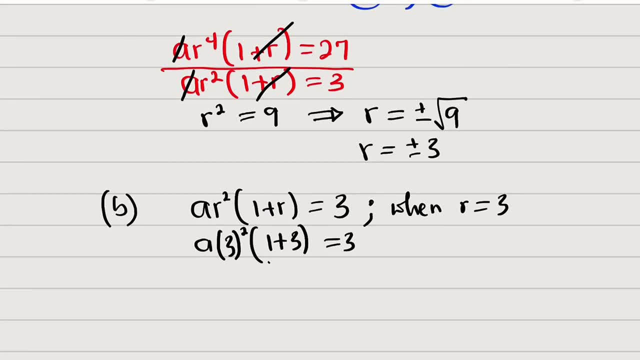 equal to 3, this is 4, this is 9. if you multiply them together, you have 36. therefore, we have 36. a equals 3. if you divide both sides by 36, you have that a, which is the first term, equals 1 over 12. okay, what if r is negative, 3? 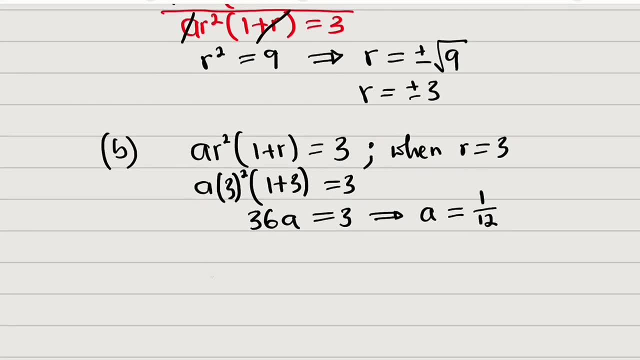 so you have a r squared multiplied by r squared, which is 3 to the second power, so you have 6. the first and third corresponds to 3, are equal to 3 minus 3. let me say, when r is equal to negative draw, we have a 3 here. 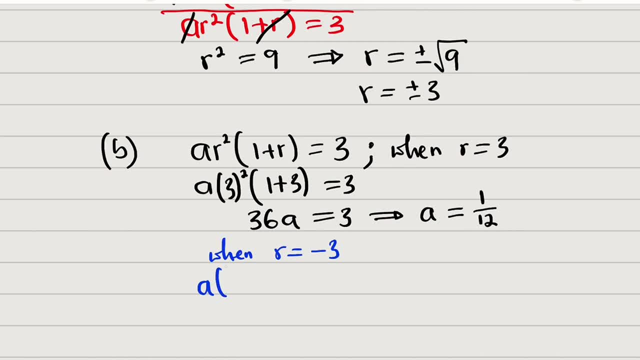 because we talked about vectors of negative draw. so in 4 i have the number of the two vectors of positive. these are the same because the��서 number of the two matrices are the same. let me say all that is equal to one. i increase or decrease this product by 1, plus or minus. 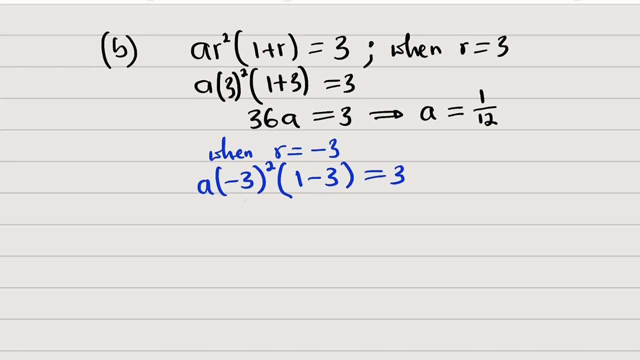 let me say when, what i will do. whenever you are smallest number, i will divide this above. This is positive 9 and this is negative 2.. Multiply together: you have negative 18.. Therefore, we have negative 18a equals 3.. 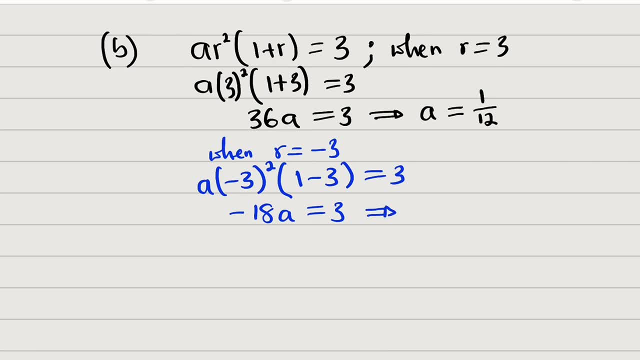 We are going to divide both sides by negative 18, and a will be equal to negative 1 over 6.. So we have two combinations here: a equals positive 1 over 12 when r is 3.. And a equals negative 1 over 6, you can see it here- when r is negative 3.. 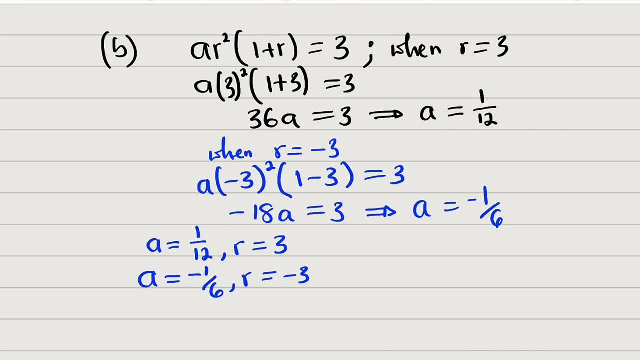 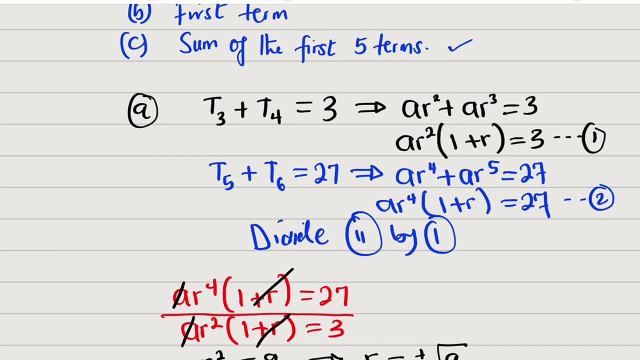 So these are the values of a with their corresponding common ratios. Now let us answer the last one, which says that we should find the sum of the factors. To find the sum of the first five times, we have to do it twice because we have to use 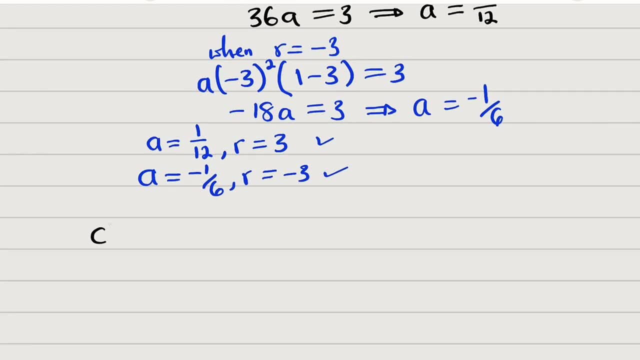 these two combinations. So we say c, the c part. we want to find the sum of the first five times when n is equal to 5,, a is equal to 1 over 12, and r is equal to 3.. Since r is positive, here we are going to use this formula. 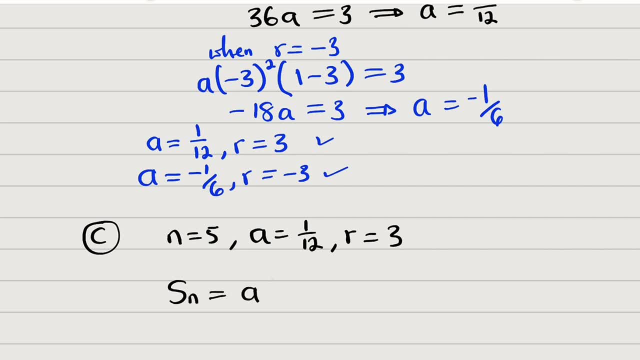 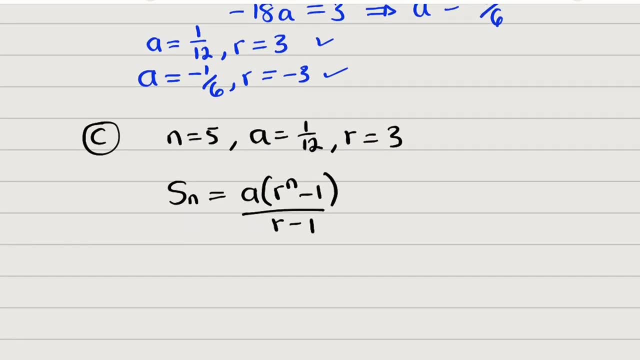 As n equals a multiplied by r, raised to the power of n minus 1, divided by r minus 1.. The substitute is 5, because n is 5 is equal to a. 1 over 12 multiplied by r is 3 raised to the power of 5 minus 1, divided by 3 minus 1.. 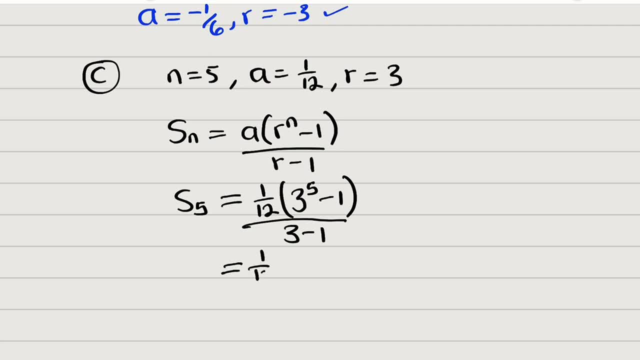 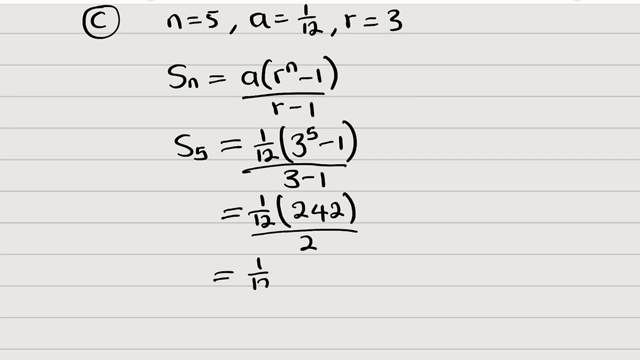 This is equal to 1 over 12.. Multiplied by 3, raised to the power of 5, is 243, and 243 minus 1 is 242.. Divide by 2, because 3 minus 1 is 2.. This is equal to 1 over 12.. 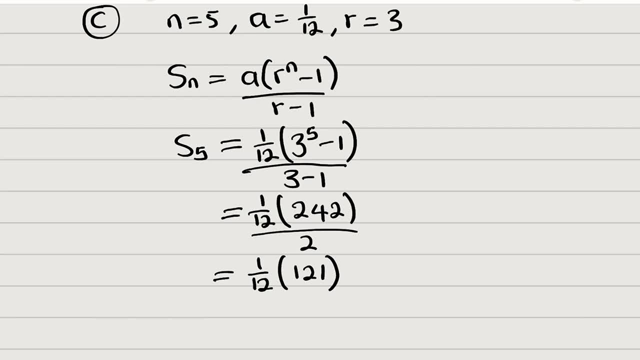 Multiplied by 1, 2, 1.. Because 242 is equal to 1 over 12.. This is equal to 1 over 12.. This is equal to 1 over 12.. 42 divided by 2 is 121.. 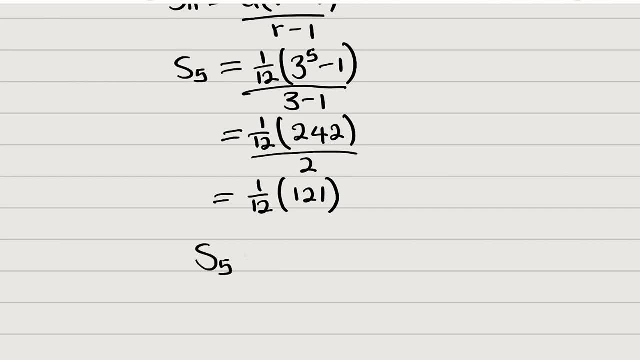 S5, sum of the first 5 times is now equal to 121 divided by 12.. And if you like, you can write it in mixed number as 10, 1 over 12.. Alright, let us look on to the other condition when A and R are both negative. 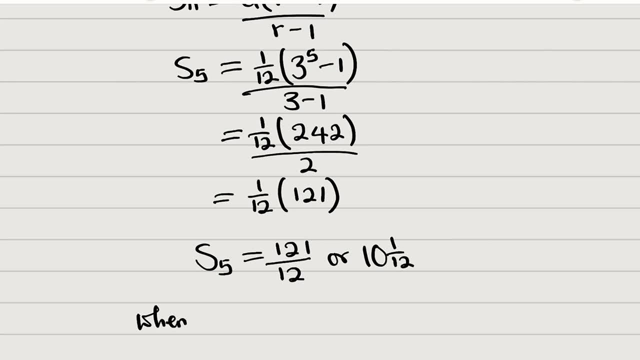 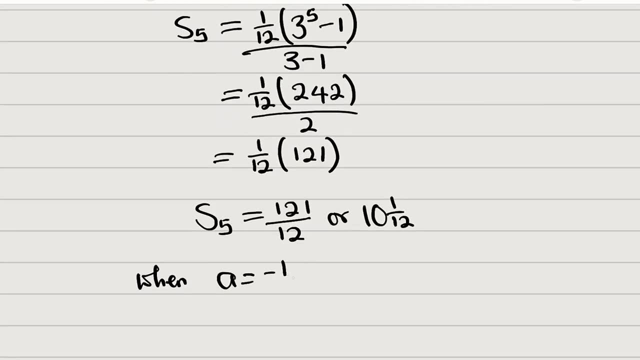 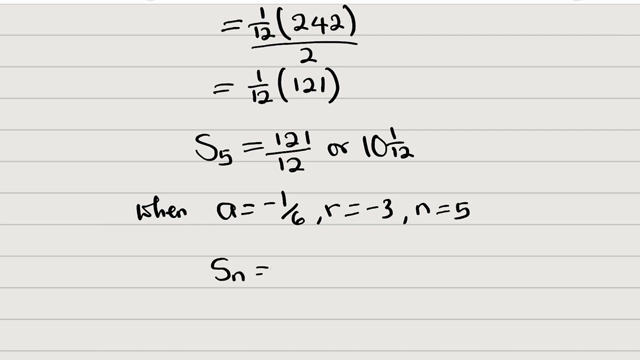 So when A is equal to negative, 1 over 6,, R is negative, 3 and remain 5.. The formula will change a little bit. We have Sn equal to A multiplied by 1, minus R to the n power divided by 2.. 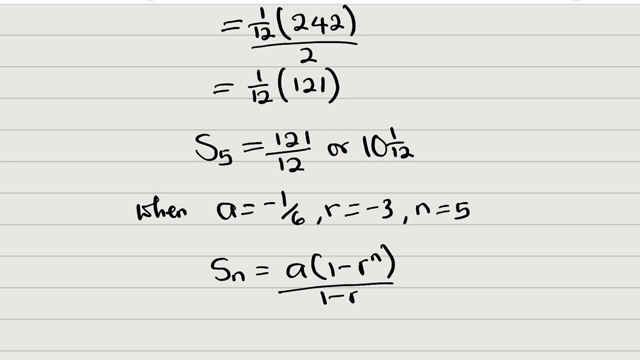 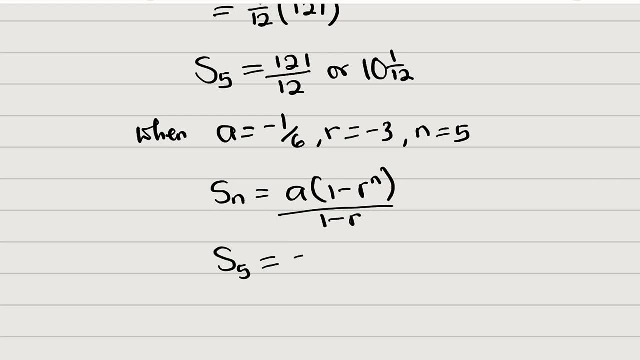 Divided by 1 minus R- Let us substitute here: S5- is now equal to A- is negative 1 over 6, multiplied by 1 minus negative 3, raised to the power of 5.. Divided by 1 minus minus 3.. 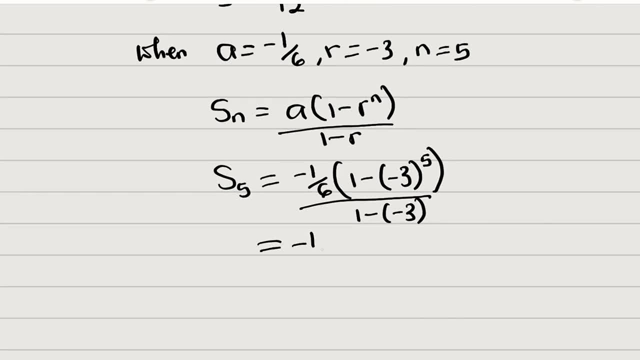 This is equal to negative 1 over 6 multiplied by 1 plus, because we have an odd power, so it will not change. 3 raised to the power of 5 is 243.. Divided by 1 minus minus 3 is 4.. 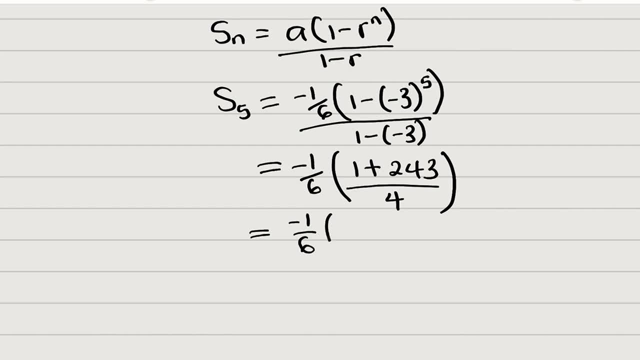 This is equal to negative 1 over 6 multiplied by 2- 4- 4 divided by 4.. This is equal to negative 1 over 6 multiplied by 6 to 1, because 2 4- 4 divided by 4 is 6 to 1..